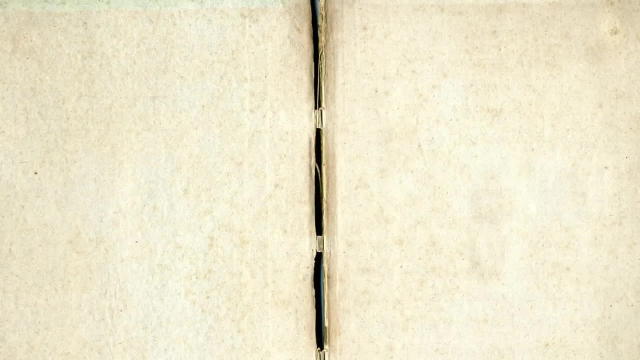 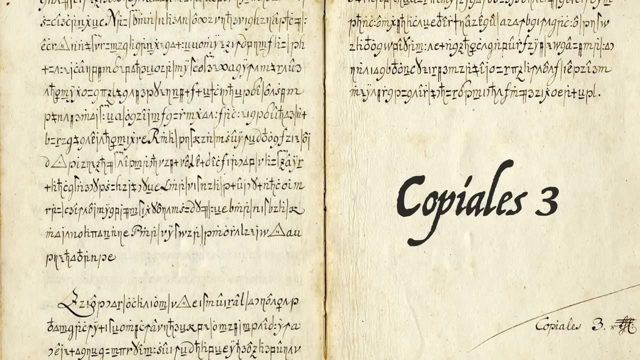 message. The only words she could read were found on the inside cover: Philip 1866, and at the end, Copiales III, a Latin word related to our word for code. The book came to be known as the Copiales Cipher. 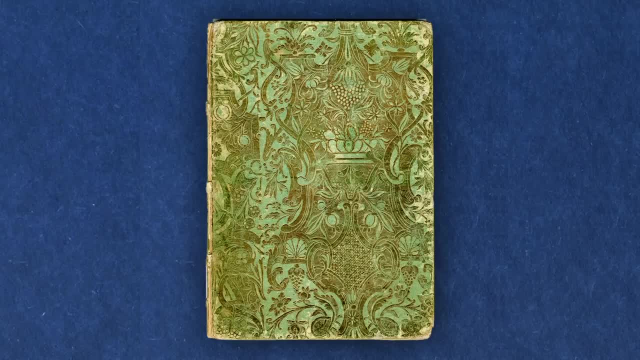 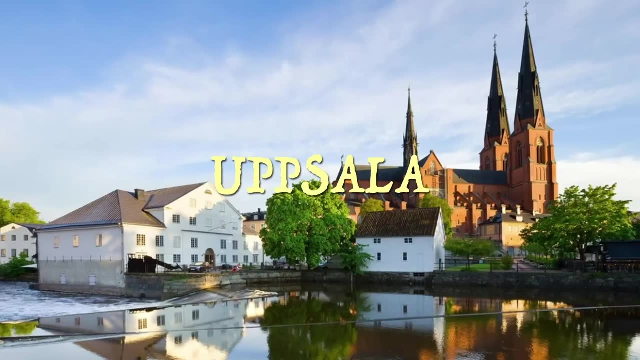 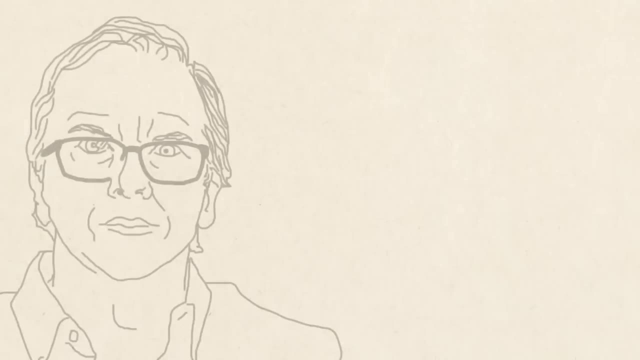 For 250 years. its message remained unknown Until 2011.. We now know what it says. Here's how it was done: Uppsala, Sweden. 13 years later, A guest speaker from the University of Southern California was visiting Dr Schaefer's university. His name was Professor Kevin Knight. He was a 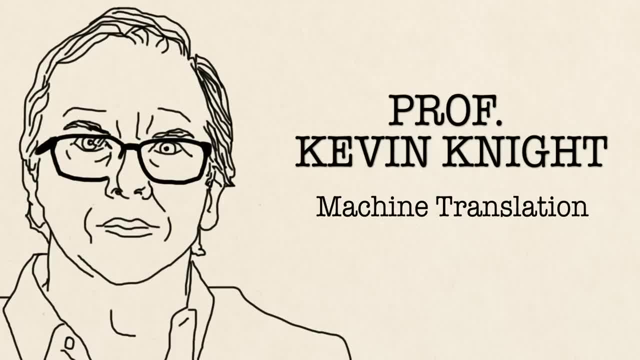 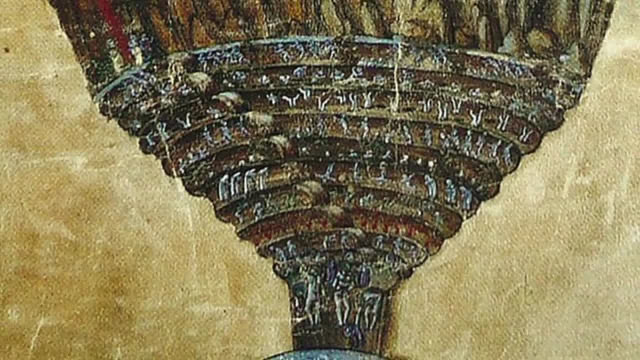 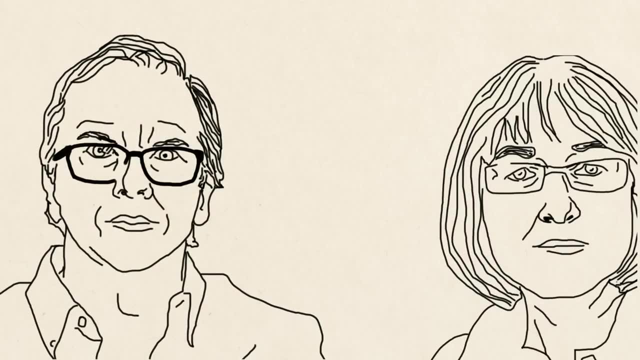 specialist in machine translation and had previously created algorithms to automatically translate one language into another, similar to systems like Google Translate. He had previously built a program that could translate Dante's Inferno based on the user's choice of meter and rhyme scheme, But he was no cryptographer. Despite this, Schaefer approached Knight with 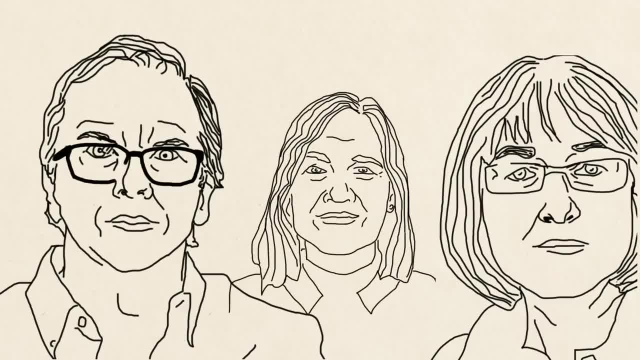 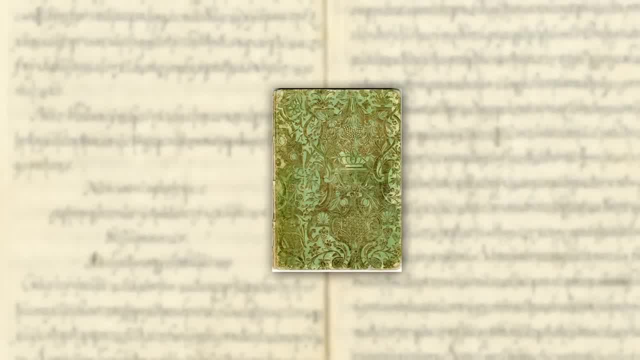 a book and the two began to discuss it Along with Schaefer's colleague at Uppsala, Beate Magiesi. the team soon began to establish that the book was indeed authentic and not a hoax. They handed the cipher to Professor Knight to take back to California and with 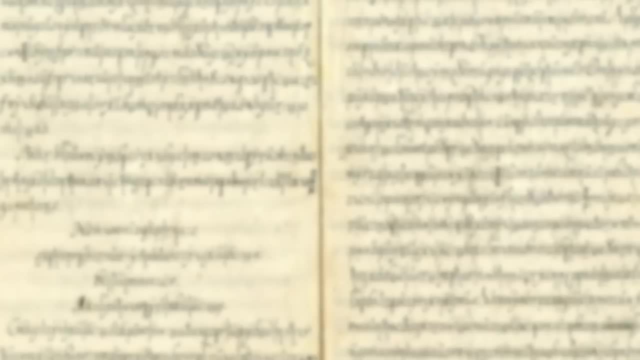 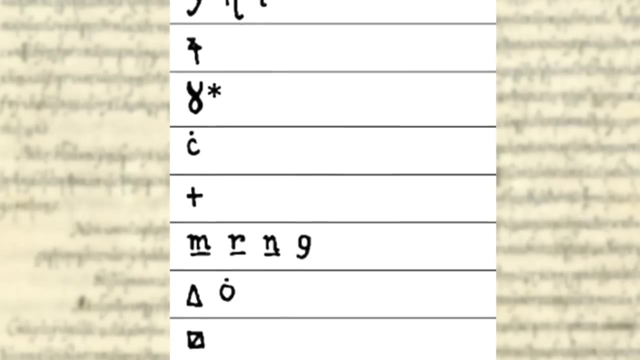 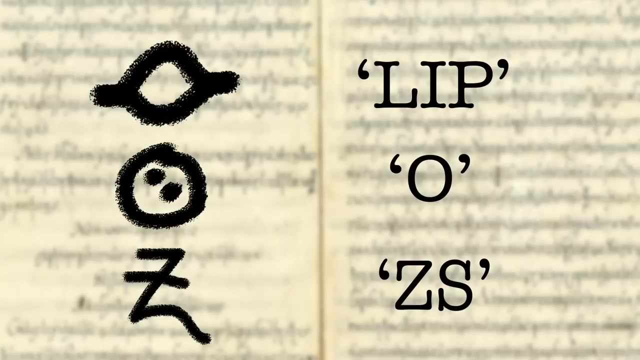 this the work began. Being a computer scientist, Knight transcribed the entire document onto a computer so it could be machine-readable. He found 88 unique symbols and gave each one a code. This symbol became LIP, this one O and this one ZS. So now, with the press of a button, the text went. 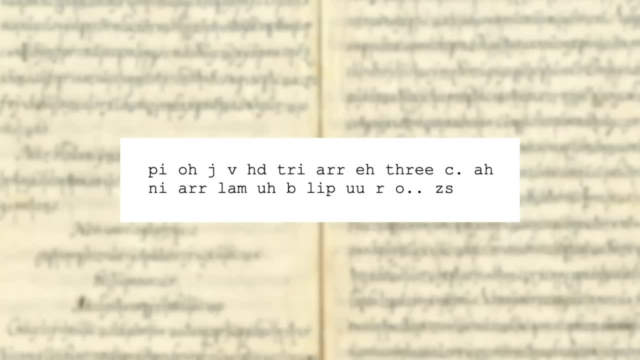 from this to this But the cipher still made no sense. But at least it was legible for his computer. This would allow him to work quickly, able to efficiently run scans to figure out any patterns or future translations. Knight first looked at the Roman letters scattered. 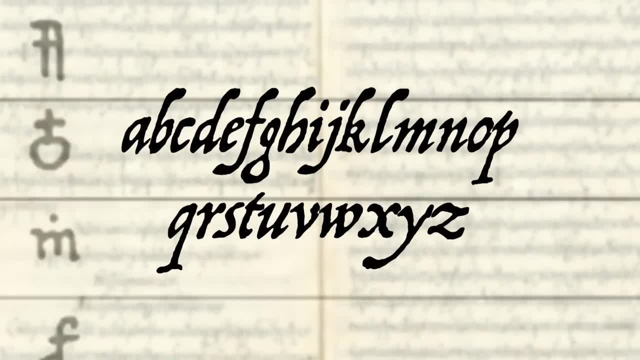 across the page. He believed that if he isolated them from the rest of the symbols, they would be able to translate them into English. This was the first time he had ever done this and he believed that if he isolated them from the rest of the symbols, he would be able to. 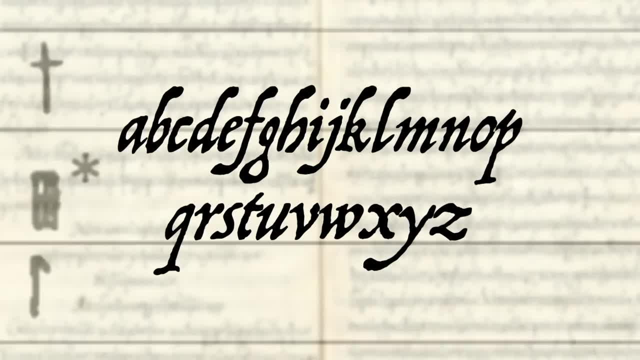 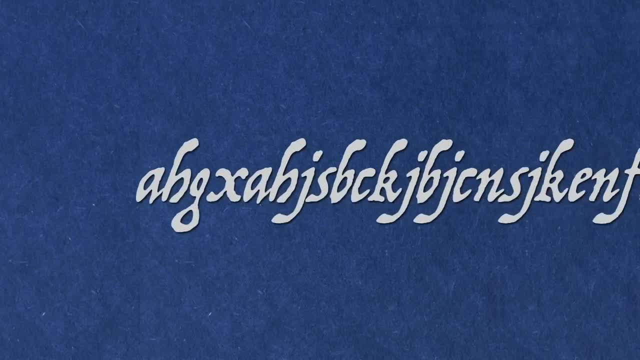 translate them into English, The message would reveal itself: In this theory, all other symbols were nulls, meaningless characters meant to throw off any cryptographers. Isolating the Roman letters did not seem to reveal much at first. They were scrambled and did not appear to have any meaning. He 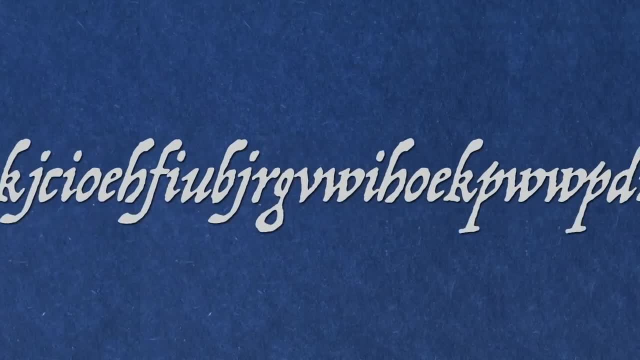 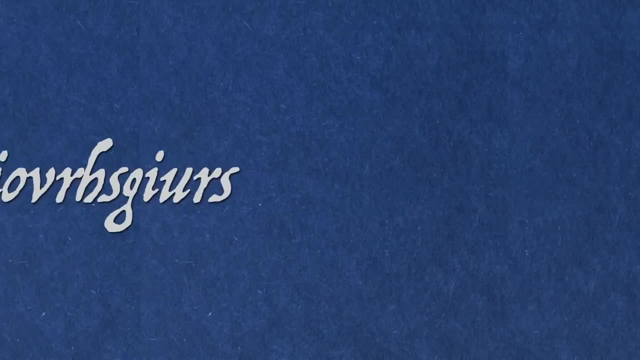 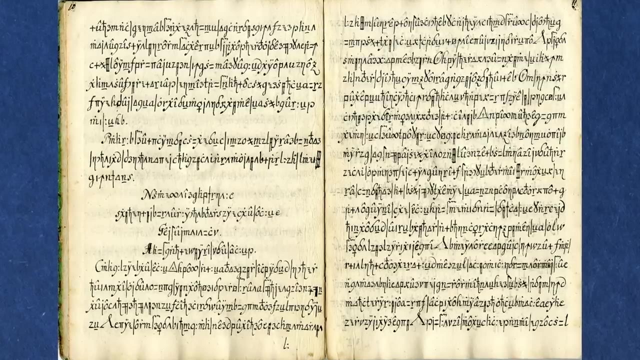 ran the Roman lettering through his databases of languages to see if any linguistic patterns emerged within the book. Nothing, The attempt was a failure and the cipher was still a mystery. Back to square one, Including all the letters. this time he ran a computer scan to see whether any letter combinations repeated themselves in the document. 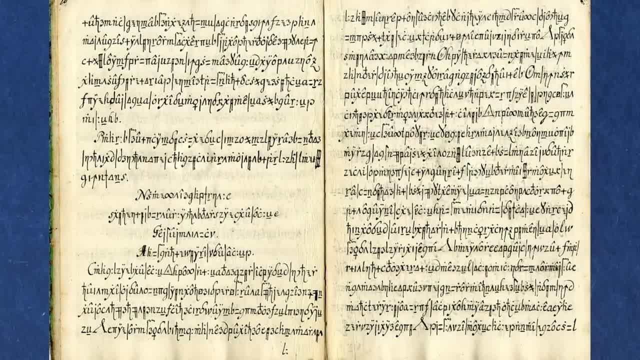 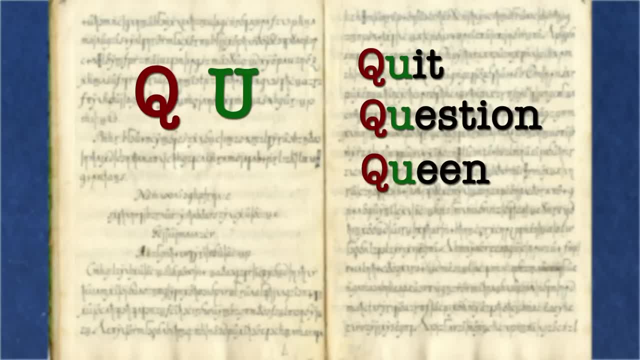 This is a smart way to figure out certain letters, as some letters only ever appear in pairs. For example, in English the letter Q is almost always followed by U Quit question: queen square acquiesce. Words like Sadiq and Fakir are of the very few exceptions, and 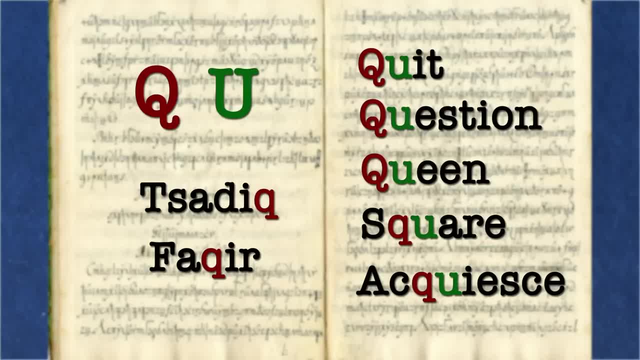 are usually imported words from other languages. If he could find unique letter pairs, it would allow him to decipher his very first letters. He ran a scan and this is the first time he had ever done this. He then ran a computer scan to see whether any letter combinations. 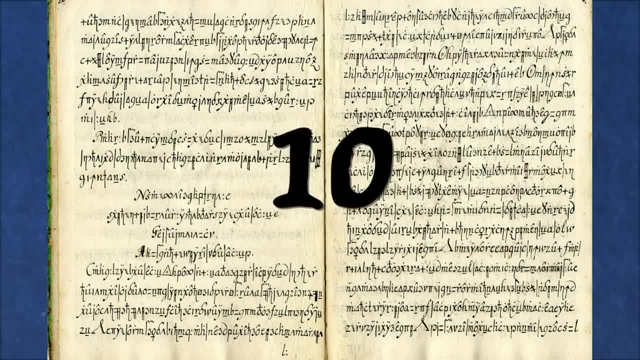 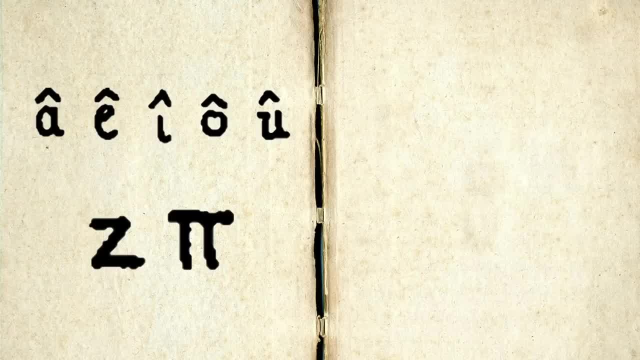 repeat themselves in the document. This is a smart way to figure out certain letters as well. There were also 10 unique character combinations in the text. It seemed that the vowels or circumflexes were frequently followed by a Z symbol or a pi symbol. This symbol was often 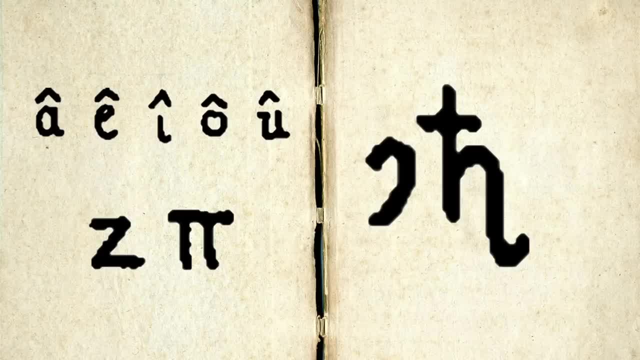 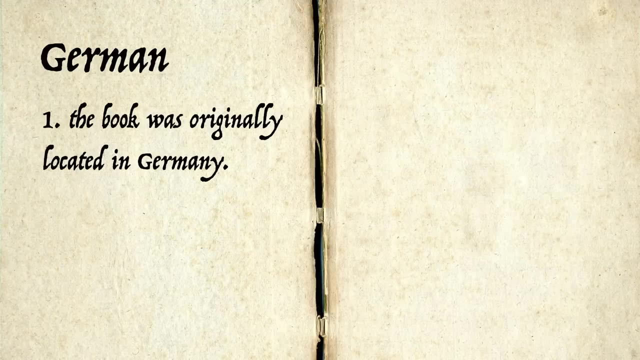 followed by this one. In some cases, this pair had a third letter form at the end. This three letter pattern would allow Professor Knight to make his first breakthrough. Knight already had reason to suspect that the original language of the document was in German. First, the book was originally located in Germany. 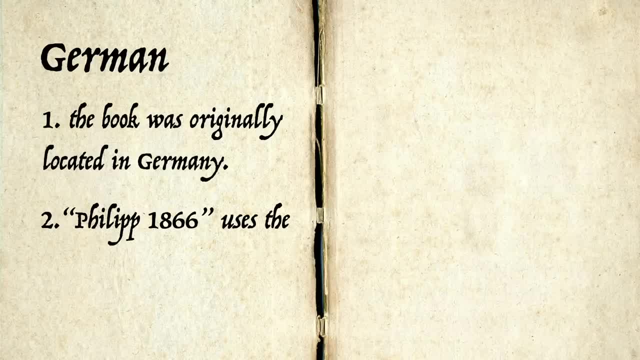 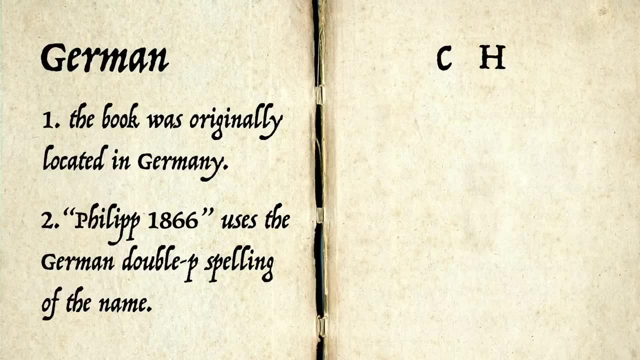 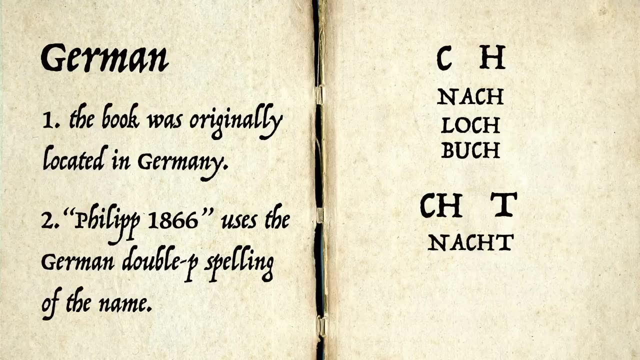 and second is the inscription Philipp 1866, which uses the German double P spelling of the name. Nightnotes says in German C was almost always followed by an H, nach loch buch, and so on. Moreover, a CH is usually followed by a T, Nacht Licht Macht. So he suspected. 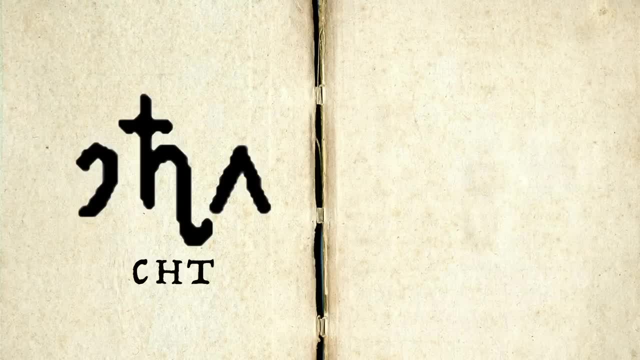 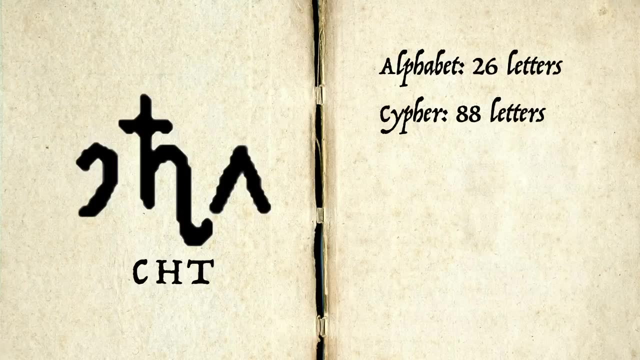 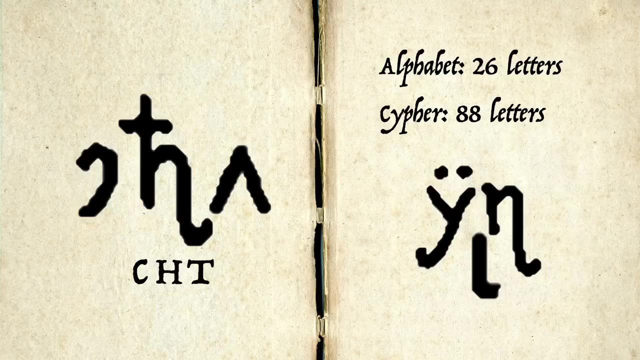 that the mysterious three letter pattern was CHT. He didn't realise it yet, but he was right. There are 26 letters in the alphabet but 88 letters in the copial. cipher Night theorised that multiple symbols must have stood for a single German letter. He played. 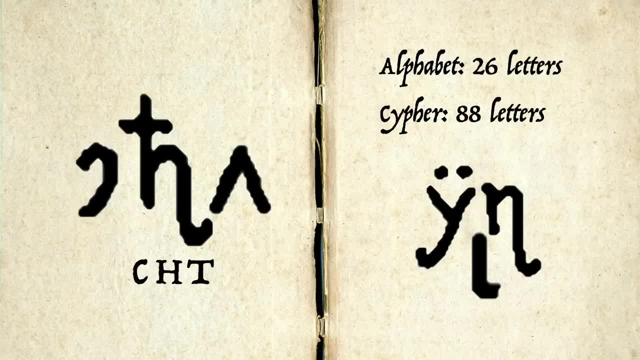 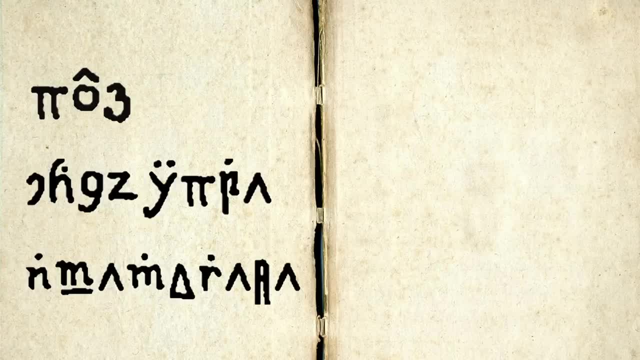 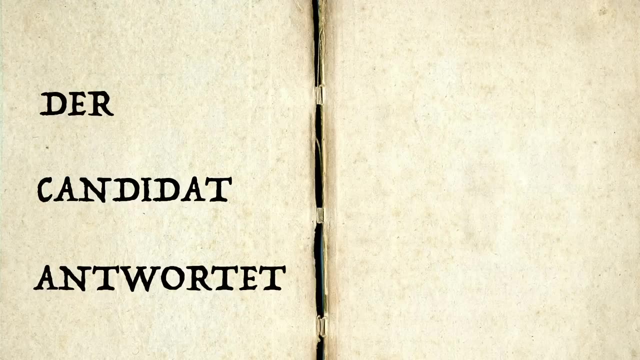 around a bit with the characters and soon discovered that these three symbols all stood for I. It seemed to work, and soon he started to assemble small words and sentences. This became der. this became kandidat. this became antwortet, Der kandidat antwortet. 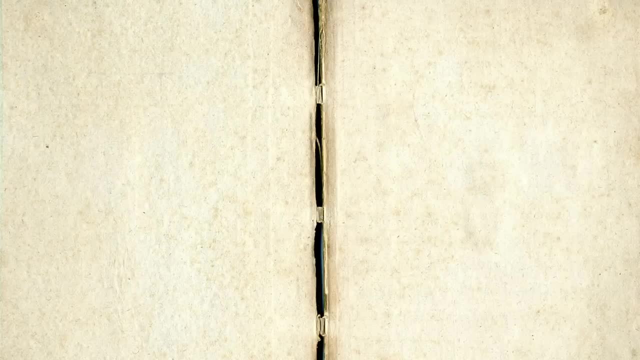 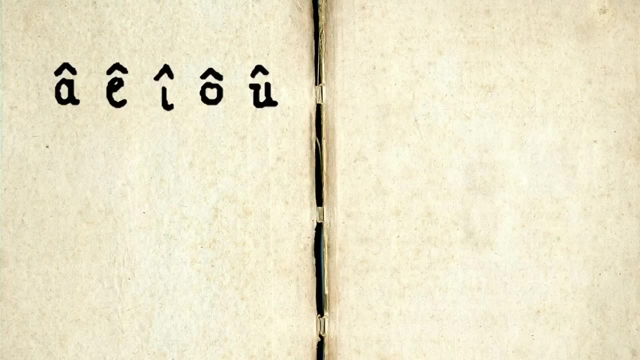 Der kandidat antwortet. This became der. this became kandidat. this became antwortet. The candidate answers. With this breakthrough, Night continued to work on the code and steadily began to decipher more and more letters and quirks. The circumflexed vowels all stood for E, This cross symbol. 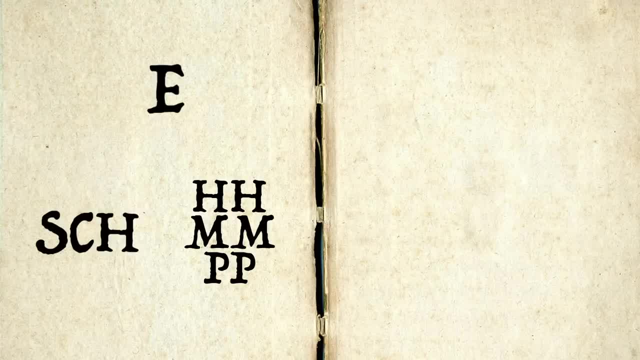 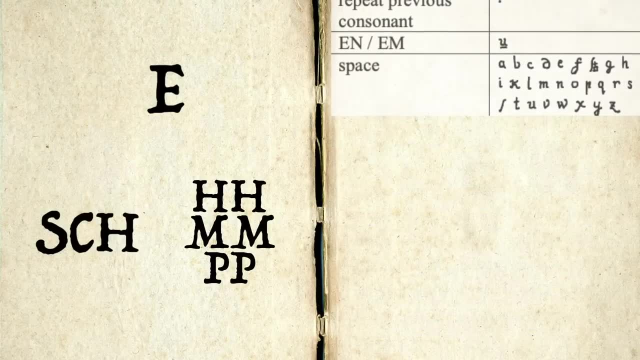 stood for SCH and the colons doubled to the previous letter. Soon Night was able to build an entire alphabet, Since he already transcribed a digital version at the start. all he needed to do was run the alphabet through his document and success. 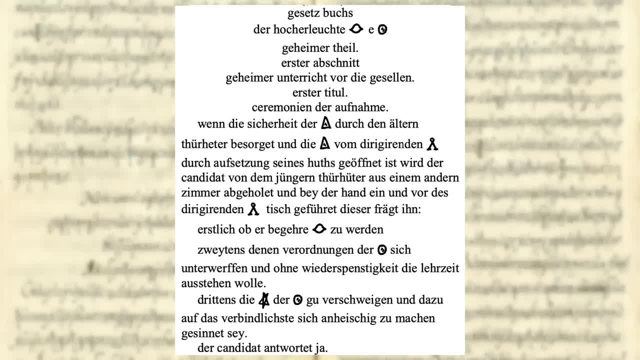 Before him lay a text that no one had been able to read for 250 years. He was right. The text was in German. What lay before Professor Night and soon Dr Schaefer and Dr Magessi, was a series. 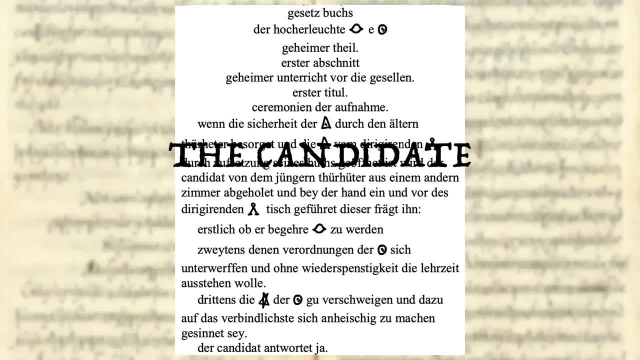 of rituals that described the initiation of the candidate into a secret group. The text is older than they thought Originally believed to be written between 1760 and 1780, it was more likely written between 1730 to 1740.. Here's the first page of the Copialis cipher. 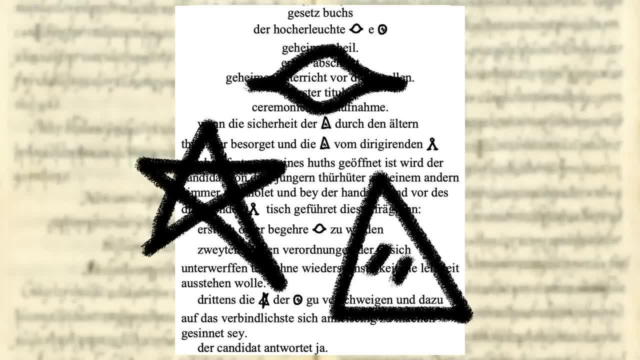 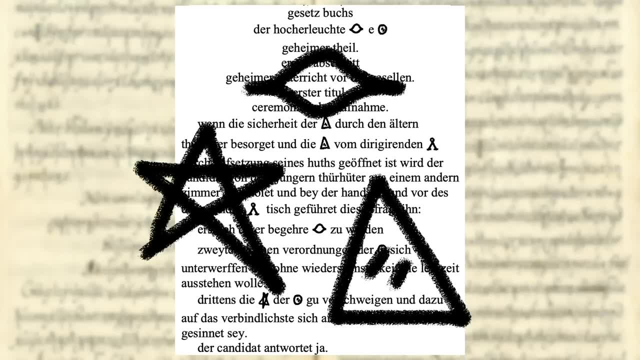 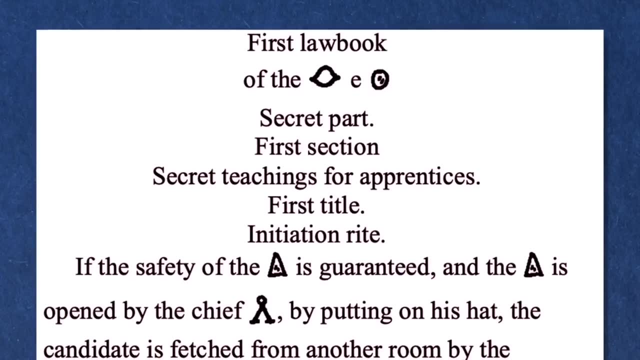 There are some large non-letter symbols yet to be decoded. The team believe that they stand in for actual names of people and roles within the organization and cannot be decoded any further. FIRST LAWBOOK OF MHN DEH IS SECRET PART – FIRST SECTION. 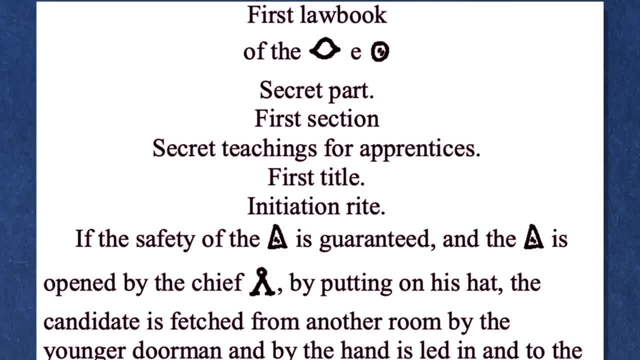 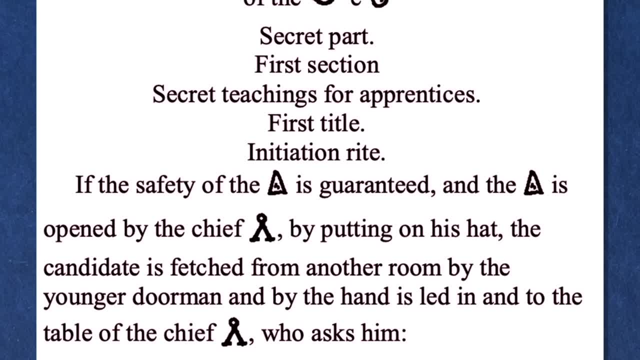 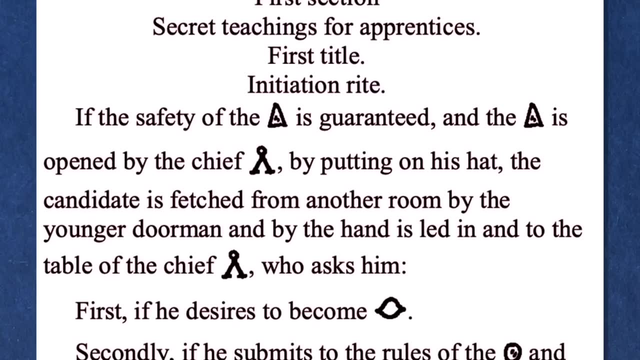 SECRET TEACHINGS FOR APPRENTICES. FIRST TITLE, INITIATION WRITE. If the safety of the is guaranteed and the is opened by the chief by putting on his hat, The candidate is fetched from another room by the younger doorman and by the hand is led in and to the table of the chief. 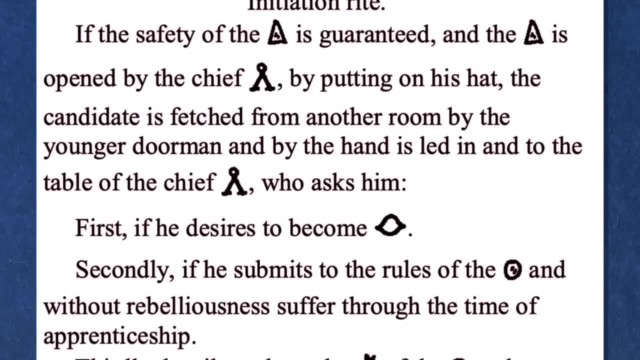 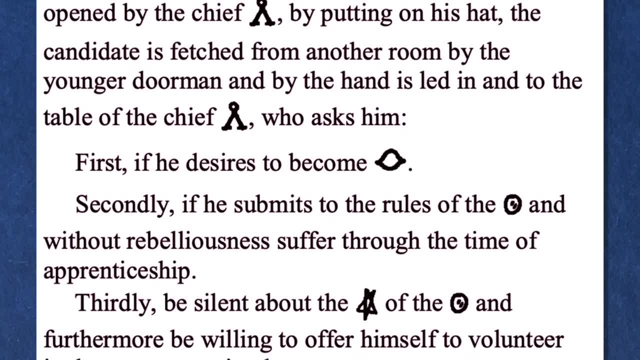 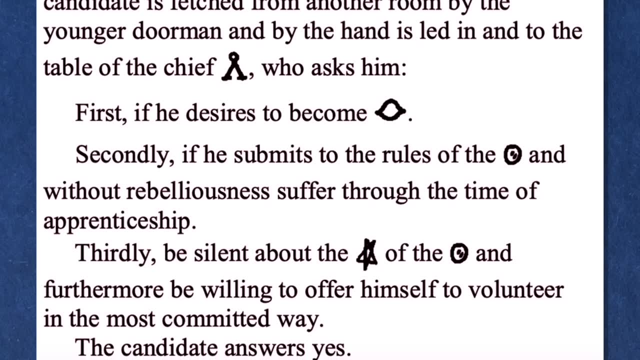 who asks him, first, if he desires to become. secondly, if he submits to the rules of the and, without rebelliousness, suffer through the time of apprenticeship. Thirdly, be silent about the and, furthermore, be willing to offer himself a volunteer in the most committed way. 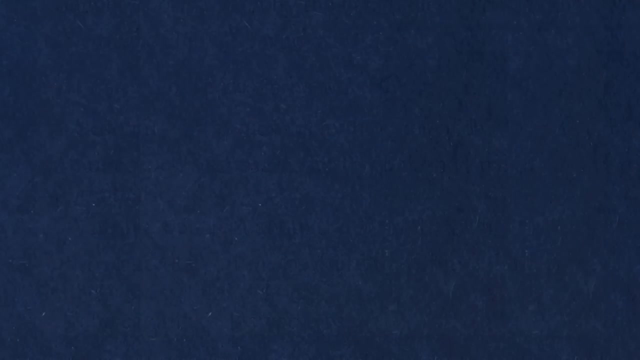 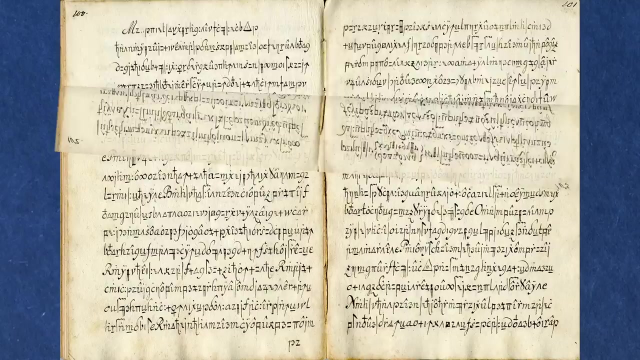 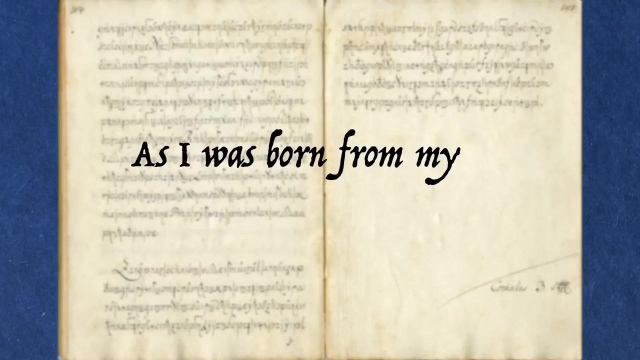 The candidate answers yes. The book continues on like this, describing complex initiation procedures and rituals, except that is for the end. The concluding pages offer a political commentary describing the natural rights of man and talks about self-evident truths: that man is born free. 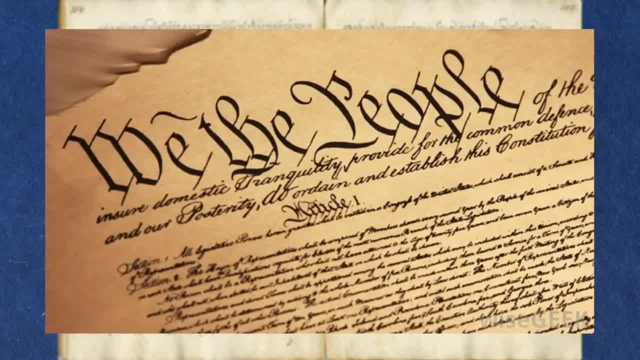 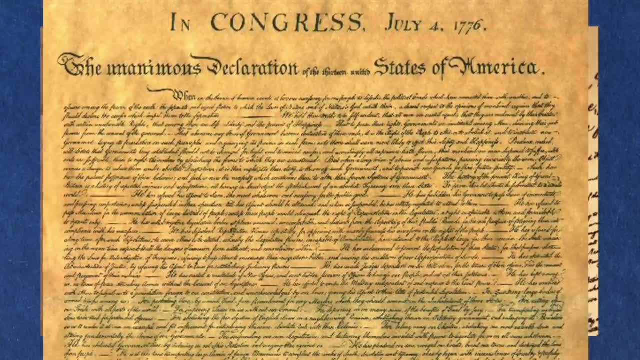 Similar language to the American Declaration of Independence, some 30 to 40 years after this document was produced, making this document one of the earliest to be espousing these sorts of ideas. But who were the authors of the document? It's never made clear in the cipher, but there are some clues. 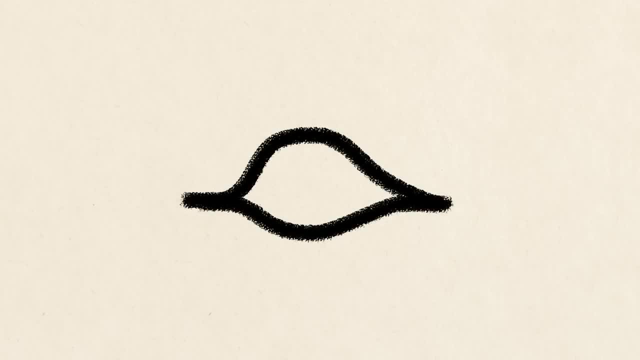 First, this symbol that appears throughout the book. It was believed to be a lip by night, but after studying it, Schaefer believed it to be an eye. Then came the recurring phrase: the light hand. This was a phrase used by German secret society known as the oculists. 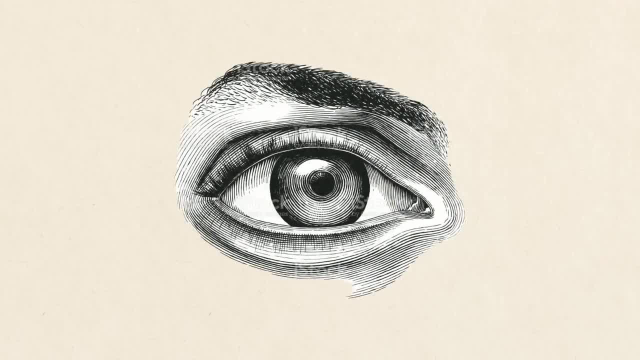 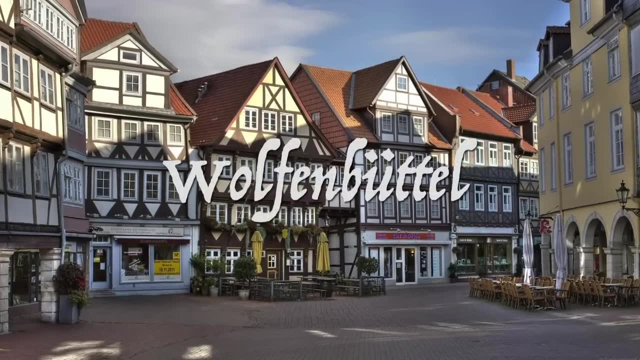 a name derived from the Latin word oculus, meaning eye. Officially known as the Great Enlightened Society of Oculists, they were based in the German town of Wulfenbudel, on the outskirts of Hanover. They were a group of academics and surgeons who performed early forms of eye surgery. 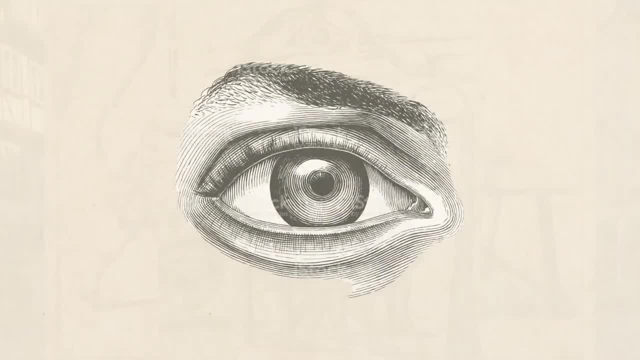 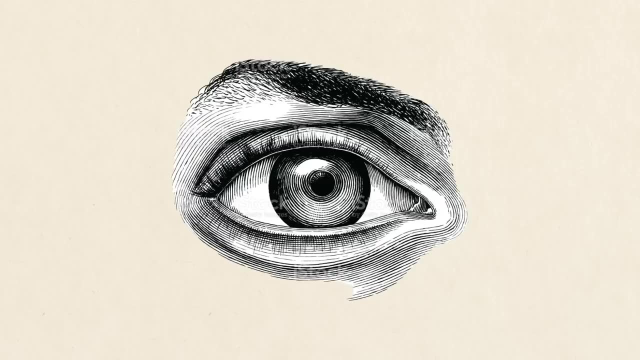 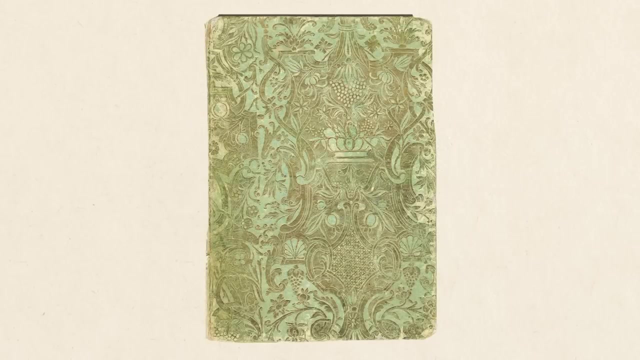 and can be recognised by their insignia featuring an eye. They were seen as being highly protective and secretive and only admitted the most respected surgeons into their organisation. This is their public image at least. The existence of a deeply complex encoded cipher implies that there was more to them than just eye surgery. 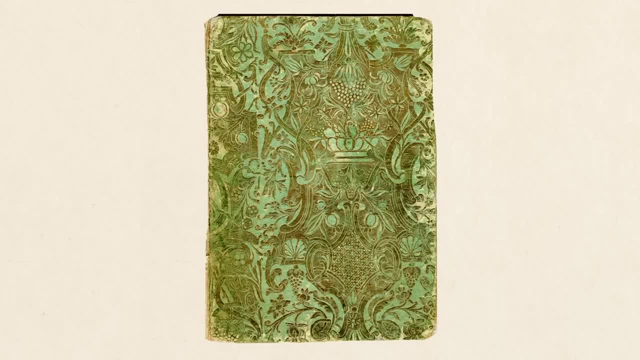 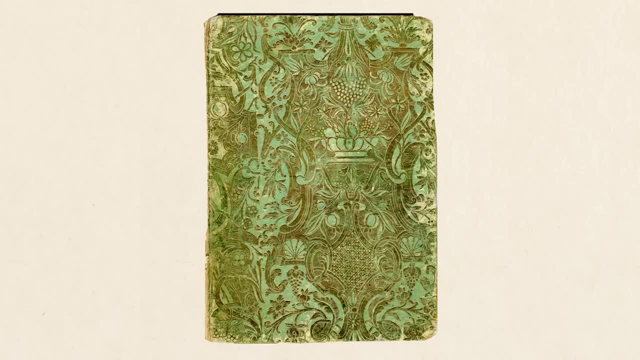 But that we just do not know. The cipher doesn't have any more information. So why the rituals? Why the political commentary at the end? What happened to the group? We know very little more about the oculists and the code of conduct. 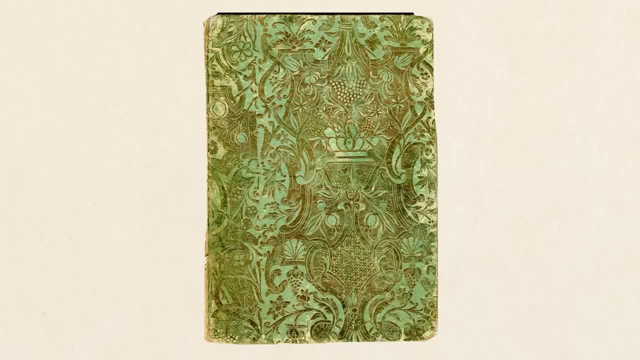 We know very little more about the oculists. We know very little more about the oculists. No, we do not know, Just pictures from Werthelzeit't. I have made another video covering reign of Rosa wyndham, with earthquakes on cervix. 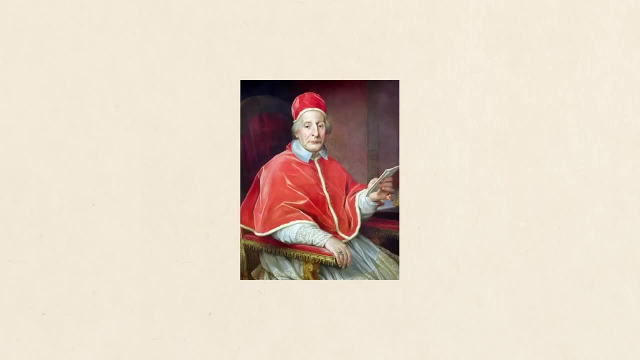 More called the Popul kilometre cipher. This is a detailed summary from the summer ofonto In September. the body size- Peterson- has remained populations. The ox shown on this photo can also be seen in this video. It is described as a Kitty cuboid.